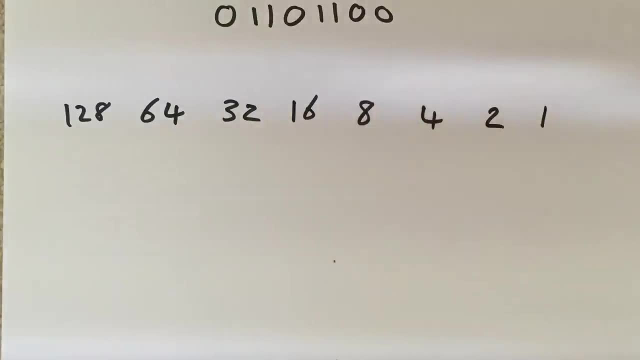 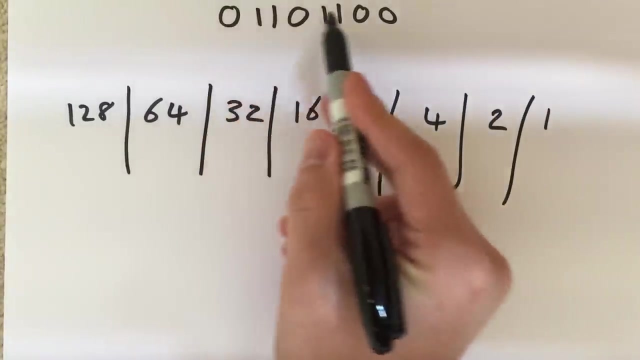 eight columns we're going to require because we've got eight digits here. Now we're going to go and write in underneath each of these columns the digits in order that they fit, and, although this might seem fairly trivial and some people will try and squeeze the numbers on top of 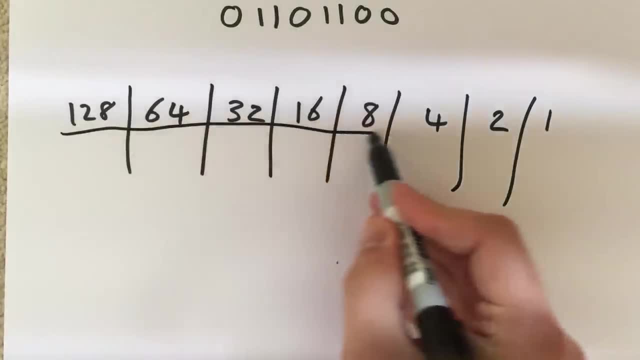 here. I think actually going through the process- spacing out clearly when you come to that crucial moment in an exam, when you need to get this right, drawing the table- is very helpful. so I'm just going to go and copy this across, and I generally start from the right-hand side sometimes. 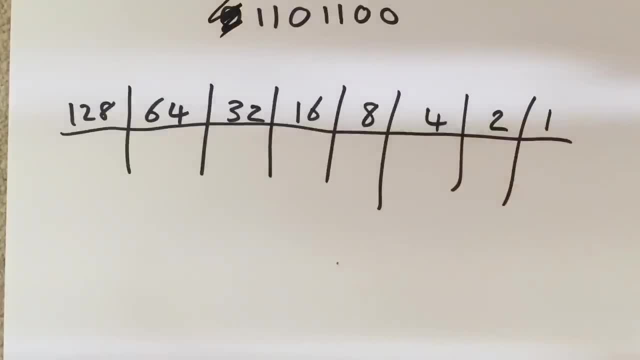 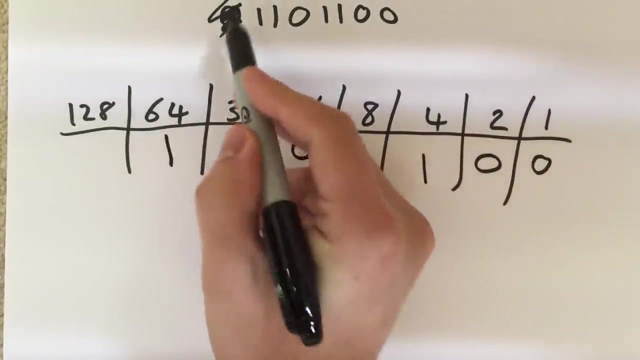 you'll be given a number without the eighth number written on it and in that situation you just assume any numbers to the left are zeros. so if you always draw from the right-hand side zero, zero, one, one, zero, one one, and assuming we hadn't been given that number, we'll just put a zero in there. 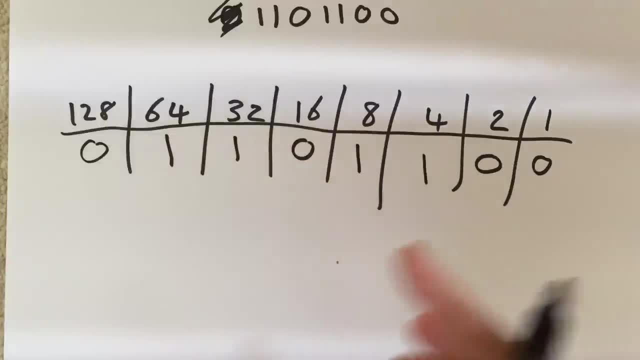 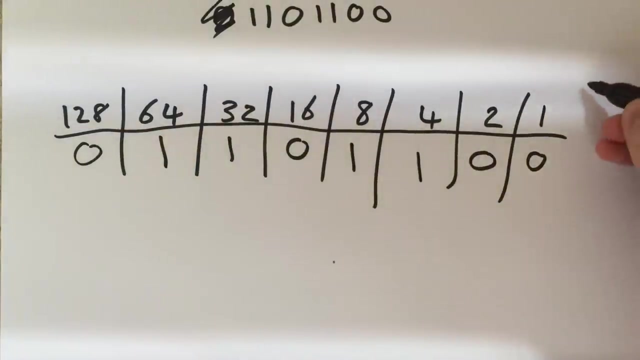 So now we can see which numbers are required and which ones are not. essentially, so, any zeros mean that we don't need that number, and any ones mean that we do need that number. so let's go and write out the number that we need here. so I'm going to start off with: do we need 128? nope, do we need 64? 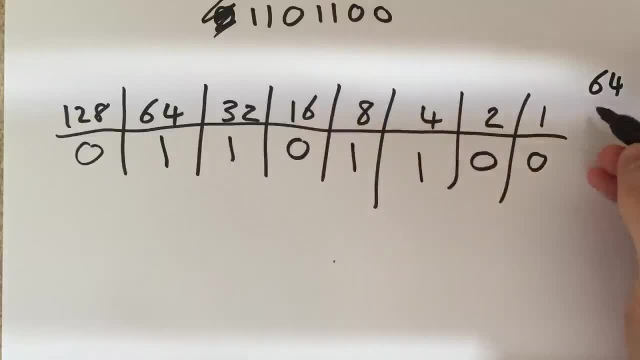 yes, so I wrote out 64. do we need 32? yes, so I'll write out 32. do I need 8? yes, notice, I'm keeping my columns here because I'm going to write out the number I'm going to write out and then I'm going to. 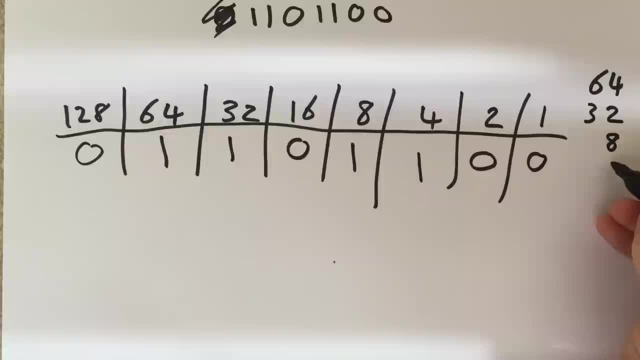 be adding these up. do I need the four? yes. do I need anything else? no, so in fact, it's just these numbers that I'm going to have to add up now. I strongly encourage you to use whatever method your maths teacher has taught you and which one you are comfortable with. we're just going to be. 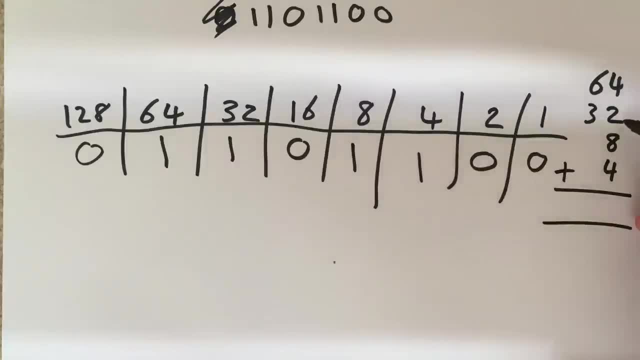 adding up those numbers now. so four add two is six. eight add six is fourteen, add the four is eighteen. carry on my one, because I'm using this method of addition. six add three is nine, add the one is ten and I've got to the answer of a hundred and eight. so now it's fair to say that the binary number 0, 1, 1, 0, 1.